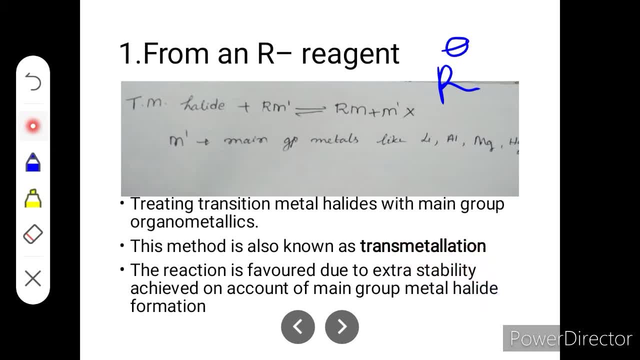 is a transmetallation reaction And this reaction is favored due to the extra stability achieved on account of main group metal halide formation Because of the formation of this M-X. this reaction is favored Because this is highly stable. M-X-N is a main group metal. 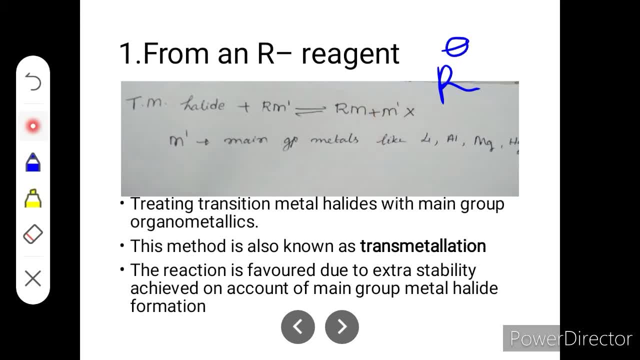 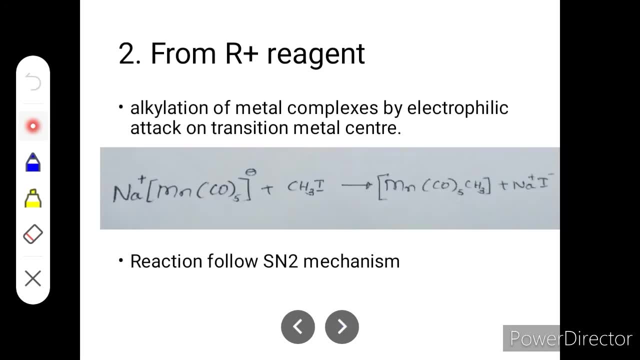 halide, That is main group metal. halide is most stable. This reaction is favored. The next method is from the R-plus region. Once again, the positive charge is on the top of this R, R-plus. R-plus means it is an electrophile. In the first method we studied about the nucleophilic. 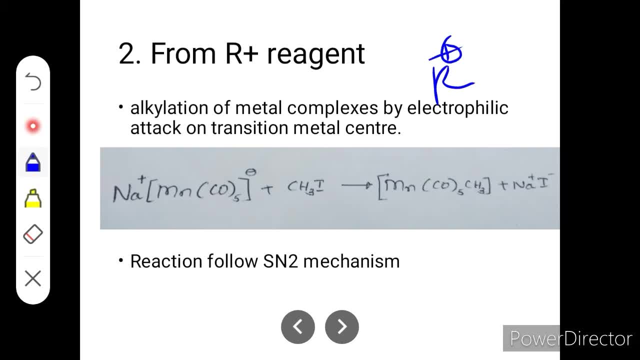 attack. Now it is an electrophilic attack. Now it is an electrophilic attack. Now it is on the metal center. Here I have given an example. Here you have the complex And this is a CH3I. So here, CH3, anyway, it will be in the positive charge, I will be in the I-. 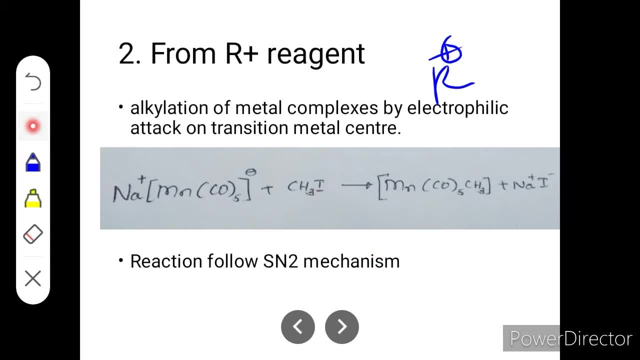 You know already CH3 plus and I minus. So here the positive charge will be present on the alkyl part. Now what happens is that the negative charge is there, This complex will be there, That will attack the alkyl Okay And the bond between the CH3. 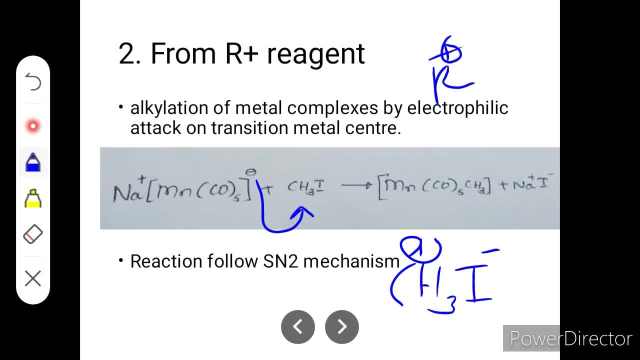 and the I. There will be a bond right between the CH3 and I And that bond will shift to the I, So I become I- So let me write here: CH3I, Right. So what happened? This negative charge will attack on the CH3 and the negative. 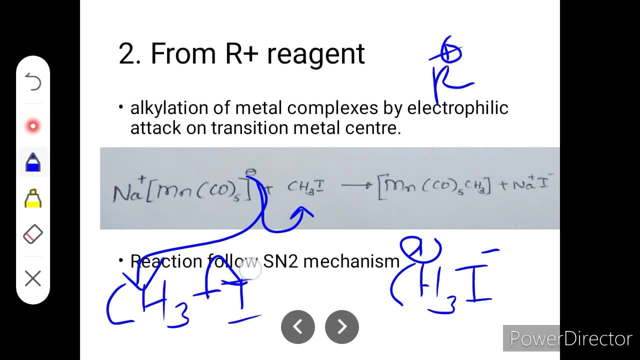 sorry, the bond between them will shift to the I And become I-. Now, here you can see this MnCO5, and along with that you will be now having the methyl part. Okay, MnCO5CH3.. Okay, And this Na- and this I- combine. 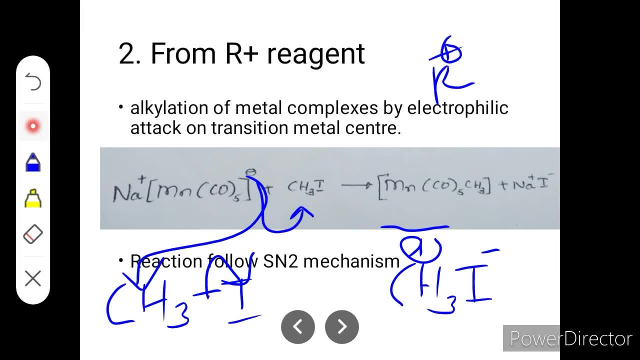 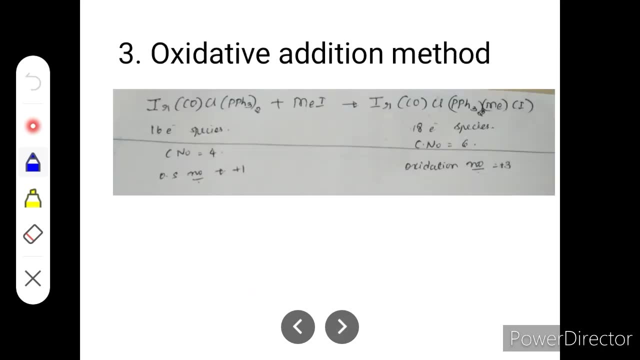 Okay, So you will see the amanine BnCO5 inhalation there. This is similar to bimmonite BnCO5 and the calcium here, where the thylactylما早 and is the monoxide in the n- dissolved state. Okay, And what we are given here now is a 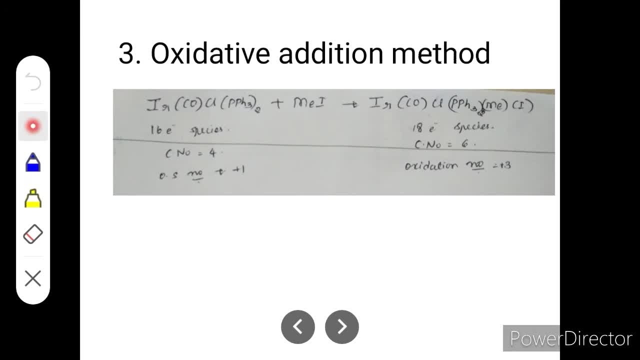 calcition. This calcination is given by saying it is the 6-isiac copper oxygen, it is converted to玉 is given. We also didn't let's say the wrought carbon lead. The ferric jedenizarium is there, Okay. 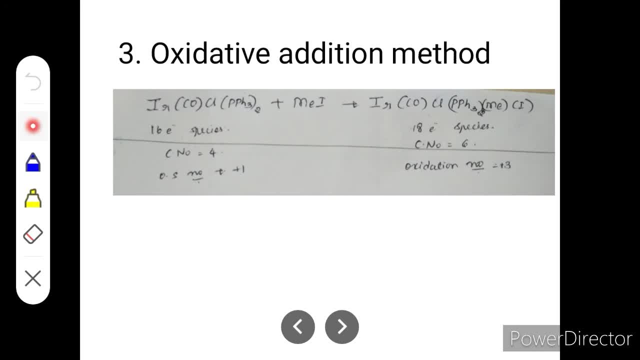 same is being taken here count by using an ionic method. In the class I explained about the covalent method and ionic method and this is calculated by means of ionic method. I have calculated by means of an ionic model method and I got the 16 electron for this particular complex. You 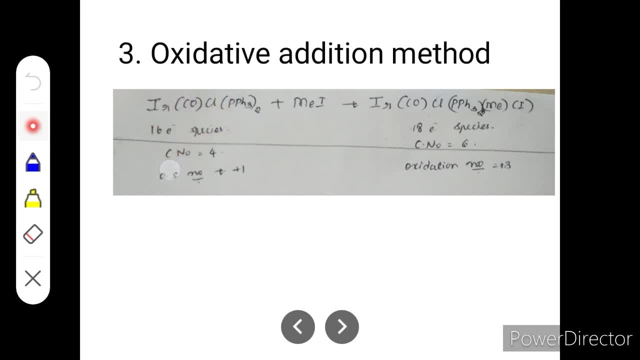 can check it by using the ionic model method, and here you can see the coordination number of this complex is 4.. This particular complex will react with the methyl iodide and you will get this product- This is your transition metal alkyl- and once again by using the ionic 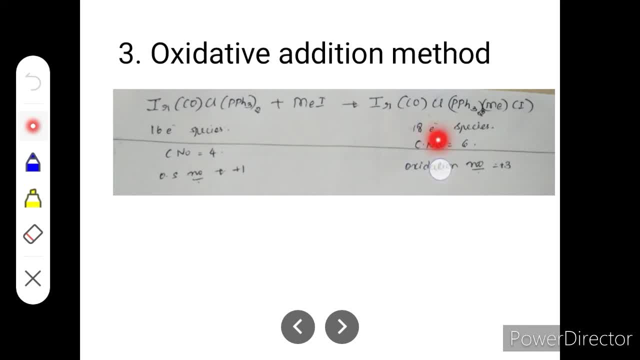 model method you can calculate the electron count. You will get the 18 electron for this particular transition metal alkyl. and for this transition metal alkyl You will get the 16 electron. and here you can note the coordination number for this is 4.. 2, 1, 1, total: 4.. Here the coordination number for the central metal atom, that is 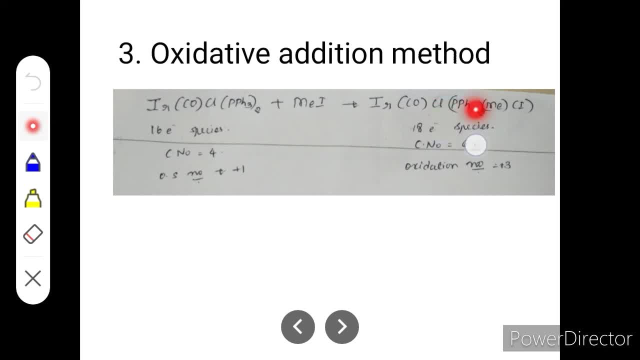 iridium is 6.. So 1,, 2, here you have. 2 means 4,, 5,, 6.. So coordination number is 6 and once again, the oxidation state of this iridium is plus 1 in this case, and it is plus 3 in. 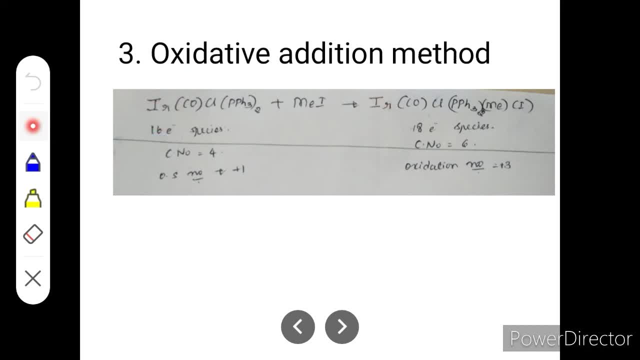 this case. So you can see. So the electron as well as the coordination number and the oxidation number in the product side is increased by these two numbers. right, It is increased by the two units. okay, The main advantage of this oxidative addition method is this method is useful for preparing.